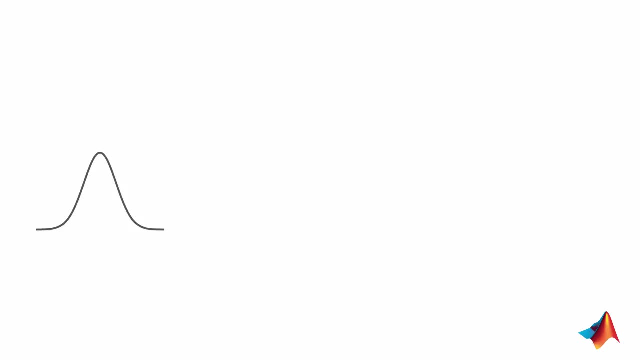 The Kalman filter assumes a Gaussian distribution. If the state transition function is linear, then after undergoing the linear transformation, the distribution maintains its Gaussian property. Although it's not shown here, the same is true for the measurement function g. However, if f is nonlinear, then the resulting state distribution 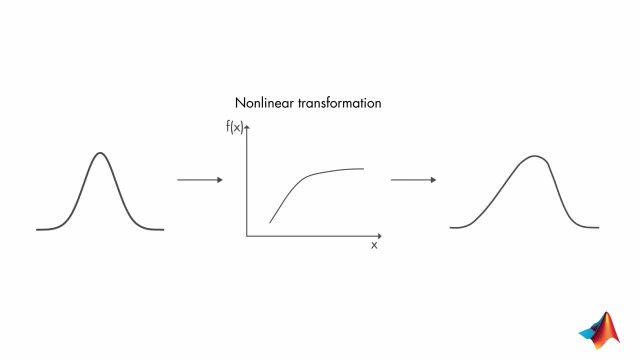 may be nonlinear. Therefore the Kalman filter algorithm may not converge. In this case you can implement an extended Kalman filter which linearizes the nonlinear function around the mean of the current state estimate At each time step. the linearization is performed locally and the resulting Jacobian matrices 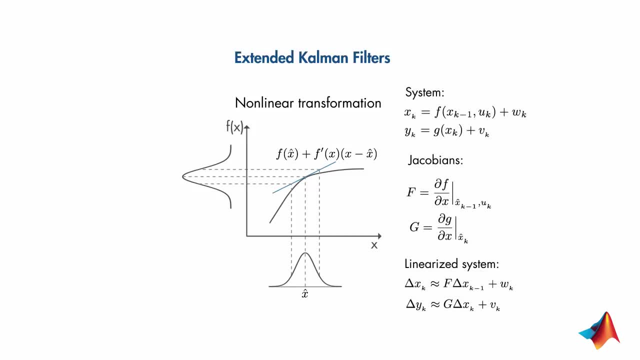 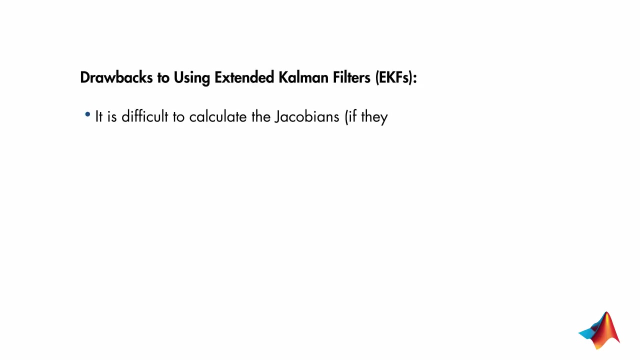 are then used in the prediction and update states. When the system is nonlinear and can be well-approximated by linearization, then extended Kalman filter is a good option for state estimation. However, it has the following drawbacks: It may be difficult to calculate the Jacobians analytically due to complicated derivatives. 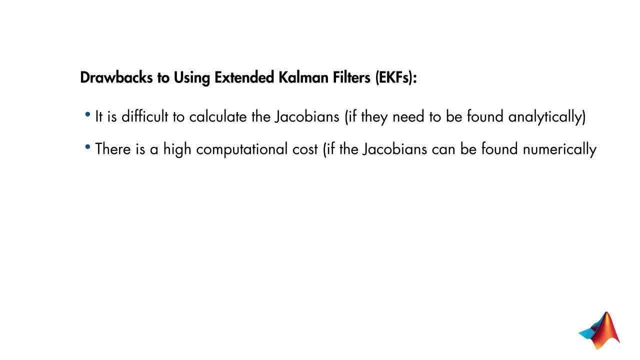 There might be a high computational cost to calculating them numerically. It may be difficult to calculate the Jacobians analytically due to complicated derivatives. There might be a high computational cost to calculating them numerically. You cannot apply an extended Kalman filter to systems with a discontinuous model, since 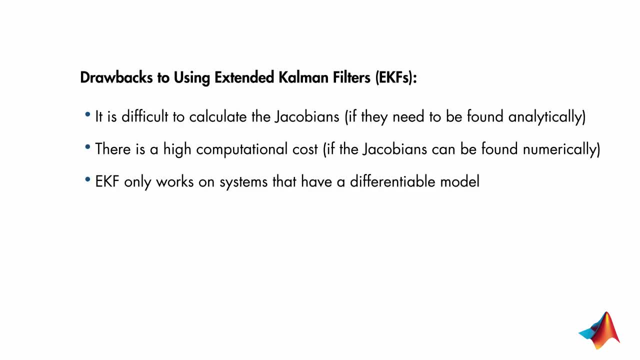 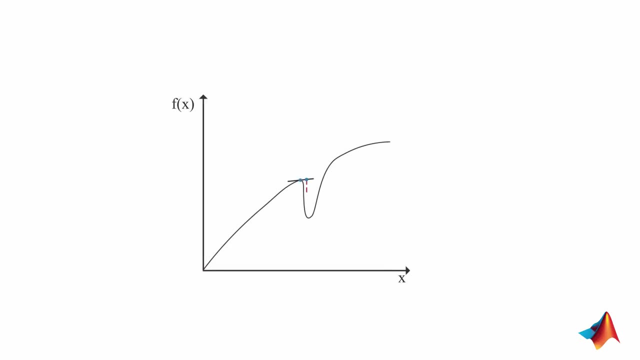 the system is not differentiable and the Jacobians wouldn't exist, And linearization doesn't provide a good approximation for highly nonlinear systems. In the last case, linearization becomes invalid since the nonlinear function cannot be approximated well enough by a linear function and doesn't describe the nonlinear function. 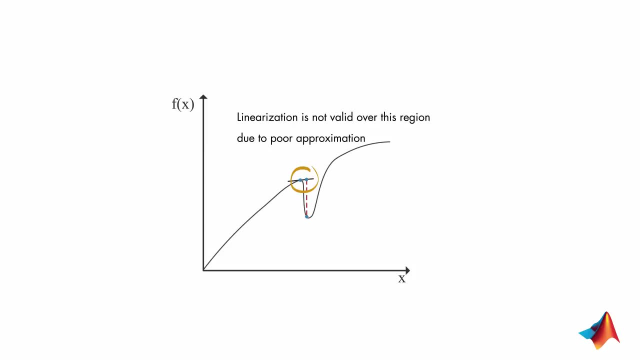 In the last case, linearization becomes invalid, since the nonlinear function cannot be approximated well enough by a linear function and doesn't describe the nonlinear function. To address the issues with extended Kalman filters, you can instead use another estimation technique called the unscented Kalman filter. 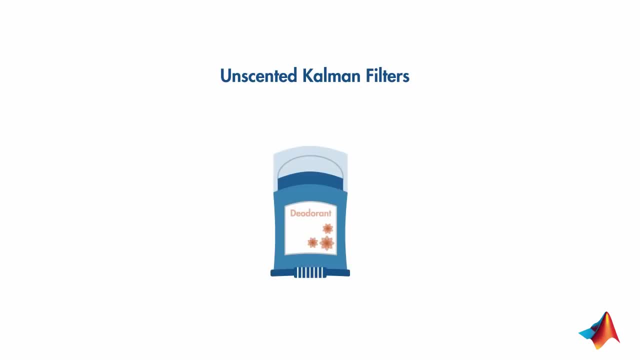 Did you know that the creator of the filter came up with this name after noticing a deodorant on his co-worker's desk? Now back to the filter. Instead of approximating a nonlinear function, as an extended Kalman filter does, we can use the unscented Kalman filter. 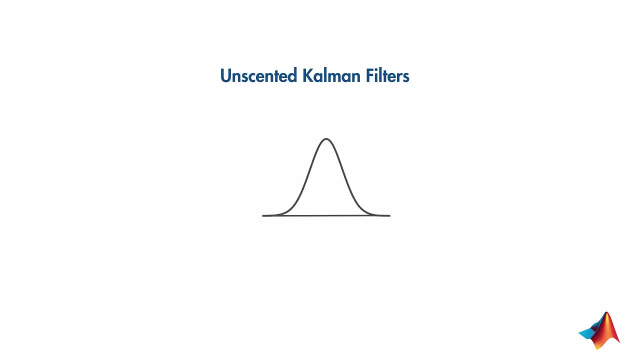 The uncentered Kalman filter is a nonlinear function. unscented Kalman filters approximate the probability distribution. What we mean by that is the following: This is a probability distribution. An unscented Kalman filter selects a minimal set of sample points, such that their mean and covariance is the same as 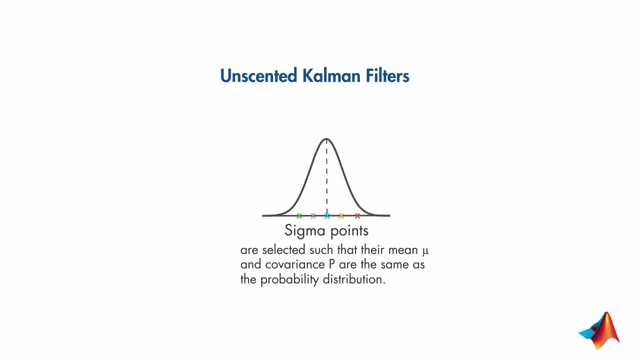 this distribution. These are referred as sigma points and are symmetrically distributed around the mean. Each sigma point is then propagated through the nonlinear system model. The mean and covariance of the nonlinearly transformed points are calculated and an empirical Gaussian distribution is computed. 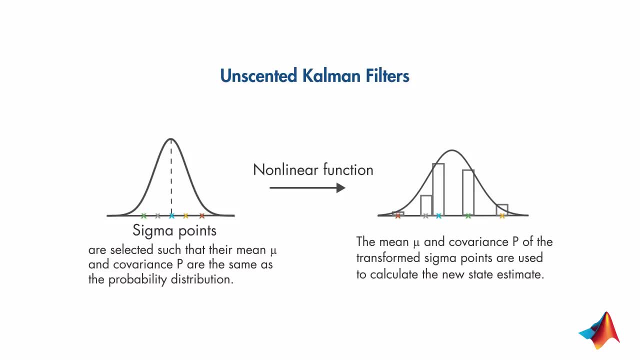 Note that in the linear kalman filter algorithm the error covariance p is calculated using Duca coefficient state transition function in the prediction step and then it is updated using the measurement. However, in the unscented Kalman filter we don't calculate it in the same way. 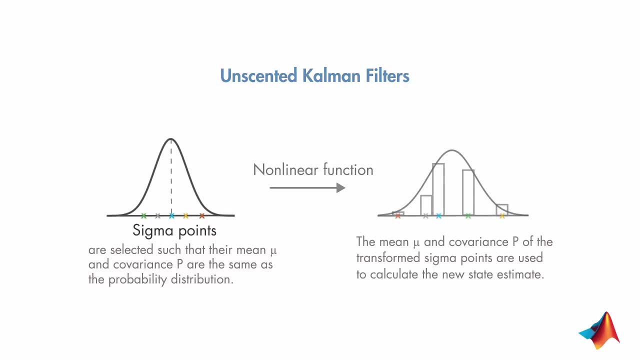 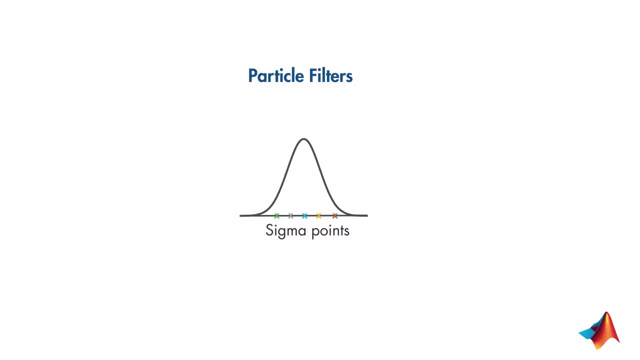 because we get it in Prickly instead. Another nonlinear state estimator based on a very similar principle is the particle filter. It also uses sample points referred as particles. The significant difference from an unscented Kalman filter is that a particle filter approximates. 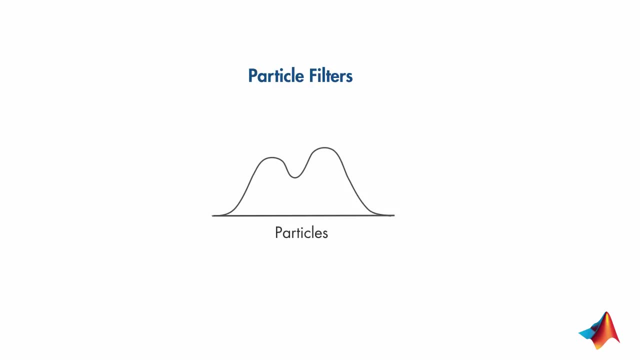 any arbitrary distribution. so it's not limited to a Gaussian assumption And to represent an arbitrary distribution that is not known explicitly. the number of particles that a particle filter needs is much larger than you'd need for an unscented Kalman filter. 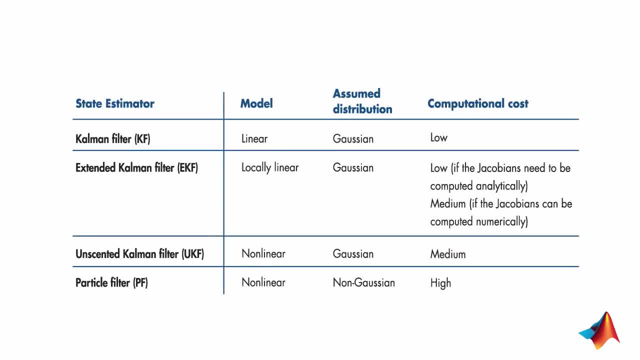 For comparison, here are the properties of the filters that we've discussed so far. A Kalman filter only works on linear systems. For state estimation of nonlinear systems you can use an EKF, UKF or PF. Note that for an EKF to precisely estimate states,